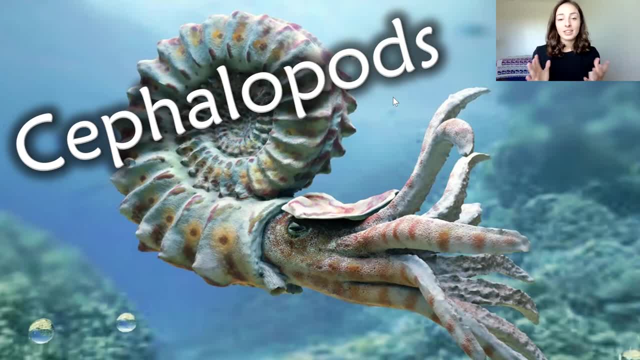 because those will help with a little bit of the background of mollusks and the entire phylum's common characteristics in general. so go check those out before we move on and if you have, then let's get started. so for some general cephalopod background information, cephalopods like i 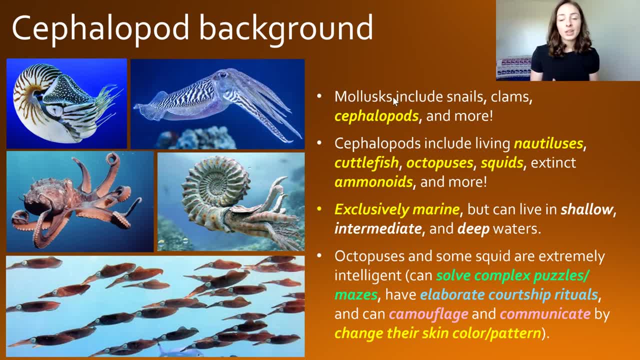 mentioned are one of the major groups of mollusks, along with snails and clams, or gastropods and bivalves, like we talked about the last video, and sometimes cephalopod shells can be mistaken for looking like gastropod shells, but cephalopods are very different than snails and we'll talk. 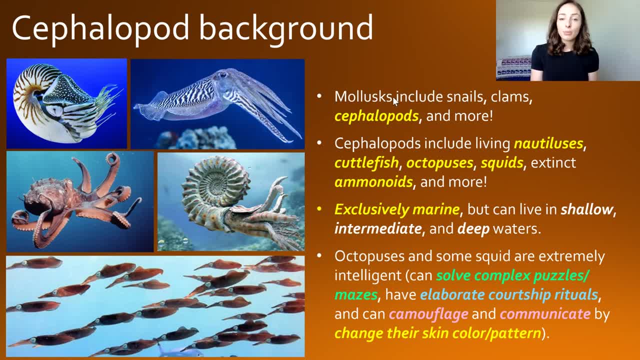 about more reasons later, but the major difference you'll see between cephalopod and gastropod shells is that cephalopods have chambers, and we'll talk about what that means later. but basically cephalopods include things like nautiluses, cuttlefish, octopuses, squids and the extinct aminoids, which, as we'll see later, are super. 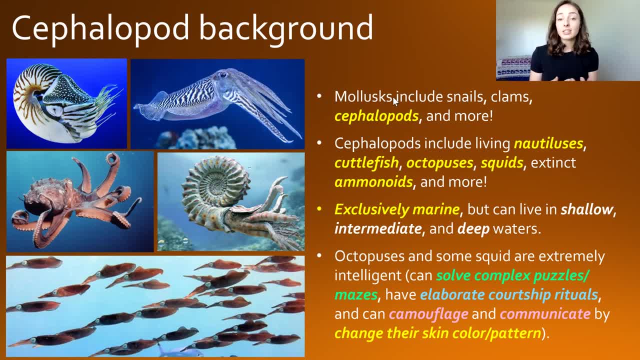 important in the fossil record. additionally, cephalopods are exclusively marine, but can be very diverse and live in shallow intermediate and very deep waters. also, some cephalopods, like octopuses for example, are very intelligent and can solve complex puzzles and mazes have elaborate. 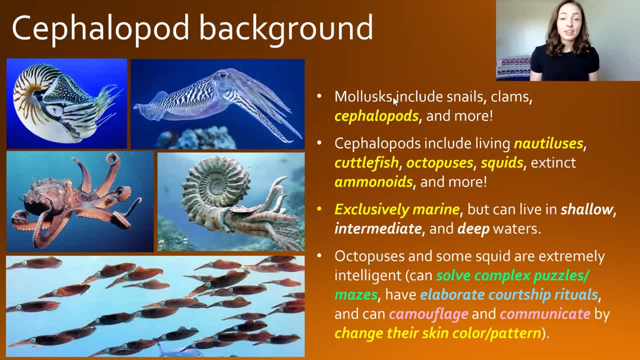 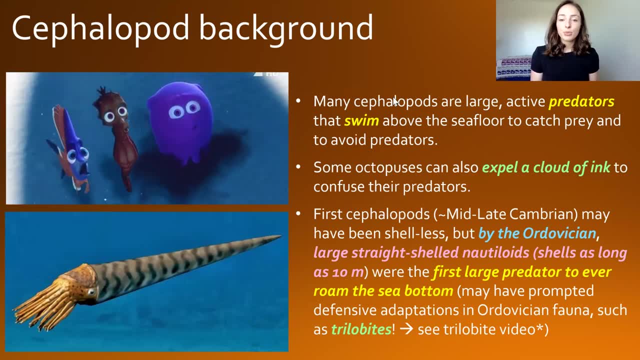 courtship rituals and can camouflage and communicate by changing the color or patterns in their skin. additionally, cephalopods are large and active predators that can swim above the sea floor to catch prey and avoid their own predators. they can also avoid their predators or confuse their predators by expelling a cloud of ink, as we can see in this little nemo gift that i show here. 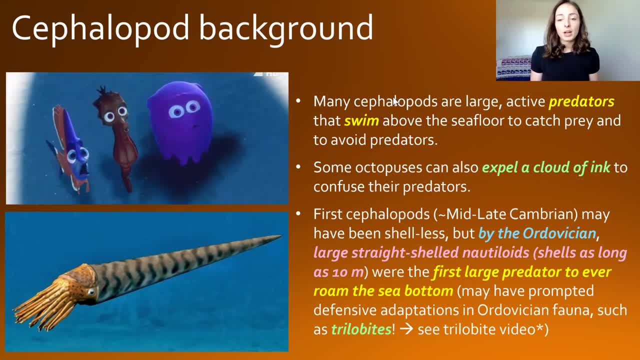 on the left and in terms of the first, most primitive cephalopods, which evolved likely in the cambrian period. they may have been shell-less, like octopuses and most squids that we see today, but by the ordovician, large, straight shelled nautiloids reaching as long as 10 meters in length were the 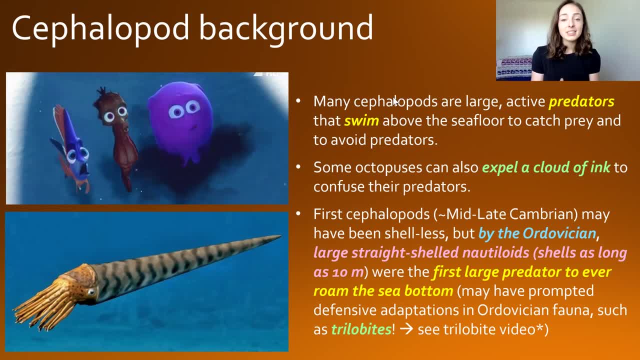 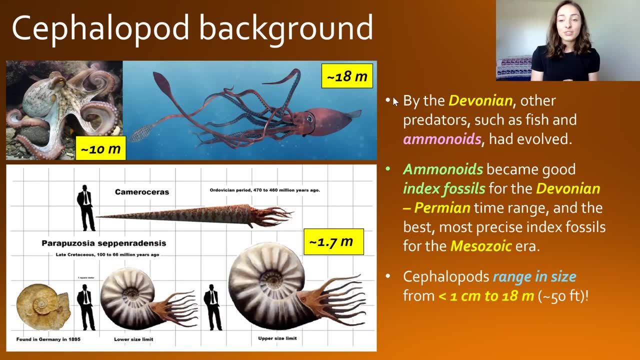 first large predators to ever roam the deep sea, and this may have prompted defensive adaptations that we see in other ordovician fauna such as the trilobites and by the devonian. other predators such as fish and aminoids had evolved to join the nautiloids in pushing. 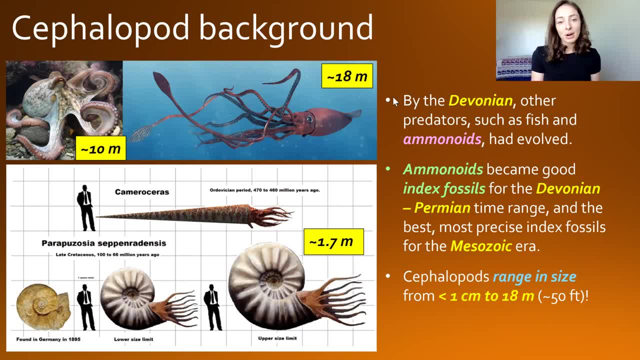 and but are also very different for reasons we'll discuss later. but basically when aminoids came on the scene, they diversified and dominated so much that they became really good index fossils for the devonian to the permian periods as well as the entire mesozoic. 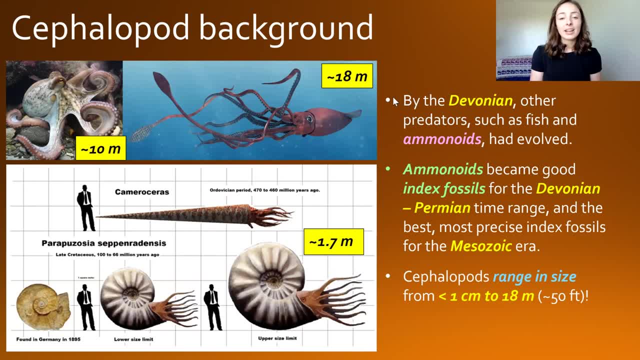 era. in fact, they are the best, most precise index fossils that can be used for the mesozoic and in of size. cephalopods like nautiluses, aminoids and squids and octopuses can range in size from less than one centimeter up to 18 meters or 50 feet in length, and we can see here that aminoids got. 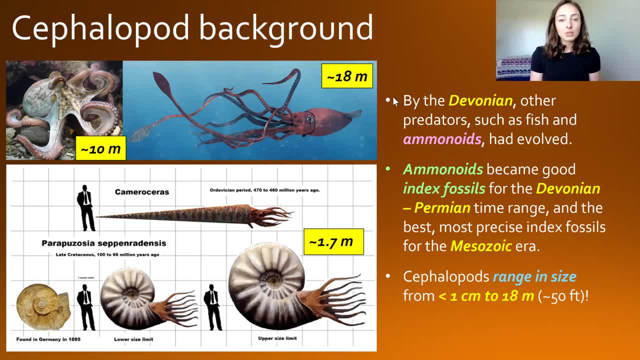 up to around 1.7 meters in size. octopuses get up to around 10 meters in size with their tentacles stretched out, but the largest cephalopod to ever have lived actually is alive today. this is the giant squid, which gets up to 18 meters in length, and this is just based on what we know from the 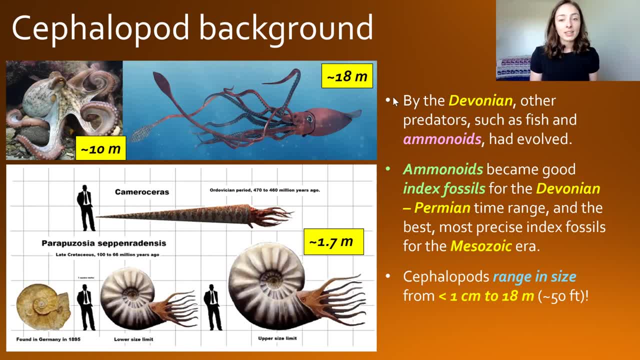 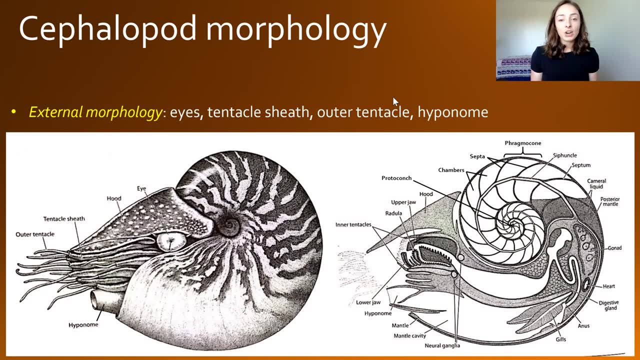 rare sightings that we actually get to see. so they might even get bigger than this and we just haven't seen it. but now that we have some of the basic background information over cephalopods out of the way, let's move on to morphology of cephalopods. here we can see that in terms of 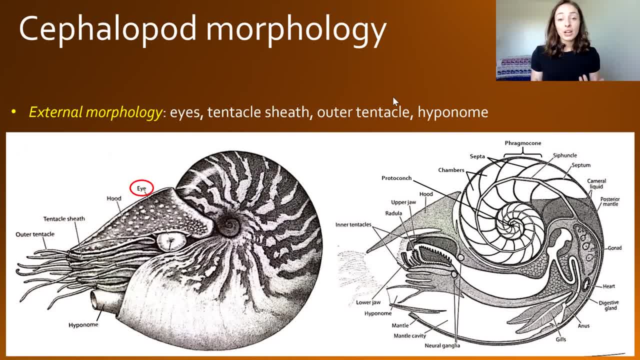 the external morphology of cephalopods. they have eyes which are actually very well developed and they are adapted to see very well in the dark so that they can go down to very far depths in the oceans, and they also have the tentacle sheath and their outer tentacles. that 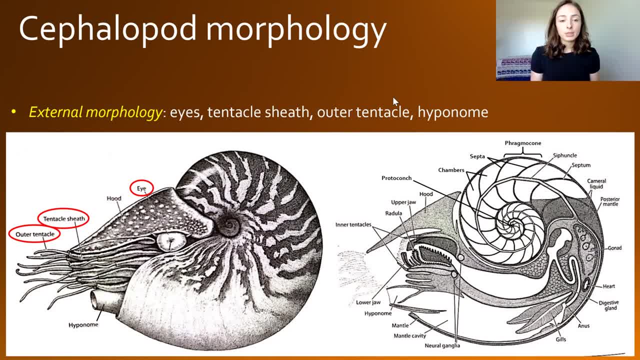 come out and grab prey or are used to maneuver themselves around. additionally, they have a hyponome, which is how they can propel themselves to swim. basically, the nautilus can flood its mantle cavity with water and then close off all the entrances and just push out all the water. 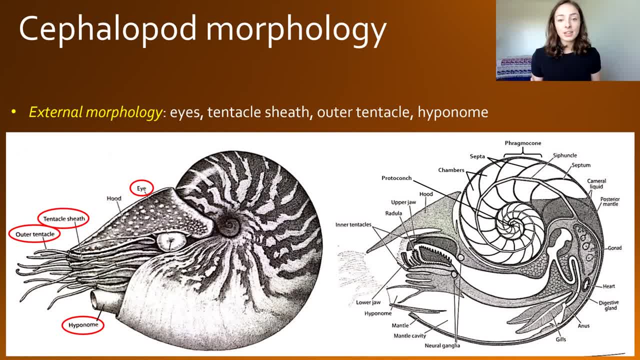 through its hyponome, causing it to propel itself backwards rapidly, and this rhythmic humping of water at the hyponome can cycle very quickly and produce rapid spurts of movement. however, this backward movement is typically only used for short-term escape and the rest of the 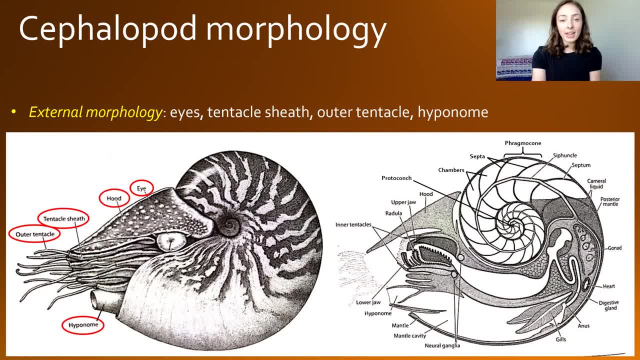 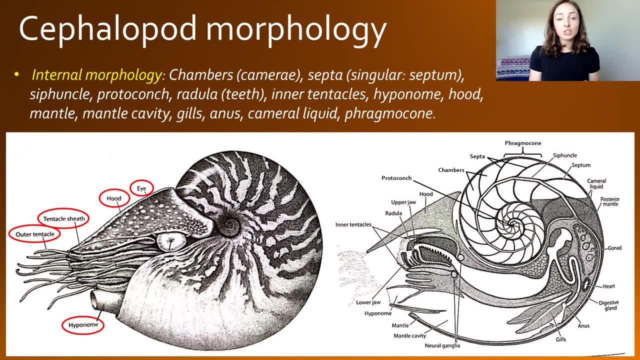 time, they typically move pretty slowly. they also have what's called a hood which can close over the body when the cephalopod wants to retract back into its shell. in terms of the internal morphology of cephalopods, they have chambers, or camerae, or camera singular, and they have septa which 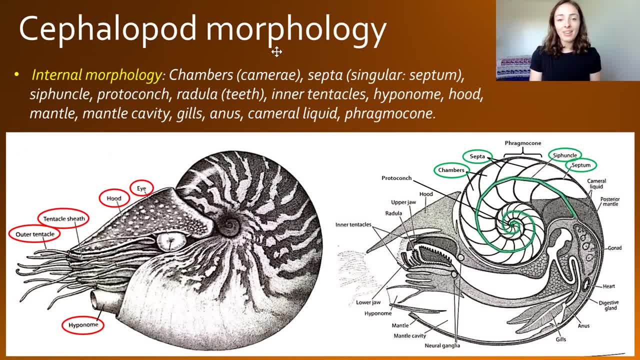 is the central part of the human body, and they also have a syphuncle, which is what's called a syphuncle, and they also have a cyfuncle, which is called a syphuncle. they divide these chambers and they also have a siphuncle, siphuncle- i'm gonna go with siphuncle, um, and this is shown by 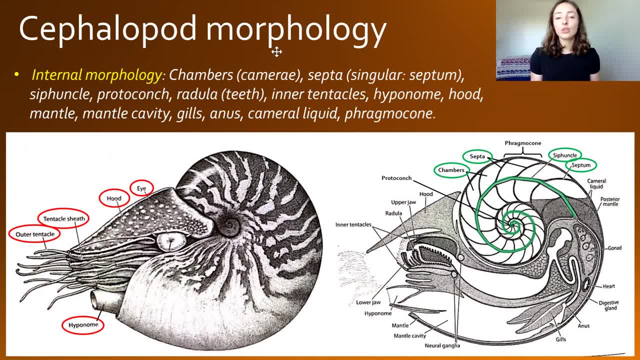 the green line here in the middle, which is a fleshy stalk that connects all of the chambers and penetrates through a hole in the center of each septum, and this feature can control the liquid and gas movement through different chambers and this helps to control the buoyancy and balance. 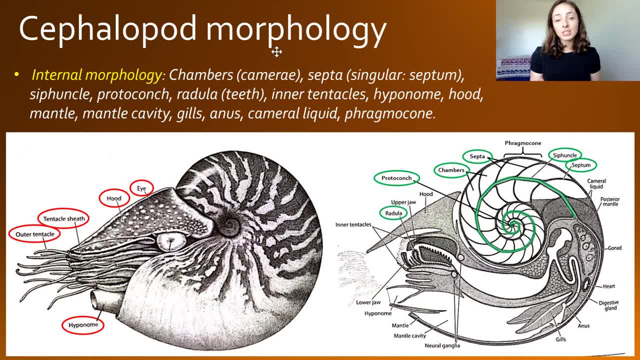 that formed, and then they also have a radula which is similar to that of snails, which i talk about in the part one monosque video, if you want to check that out. also. they have inner tentacles and then also the hyponome again is labeled here, and then they have the hood labeled again here. 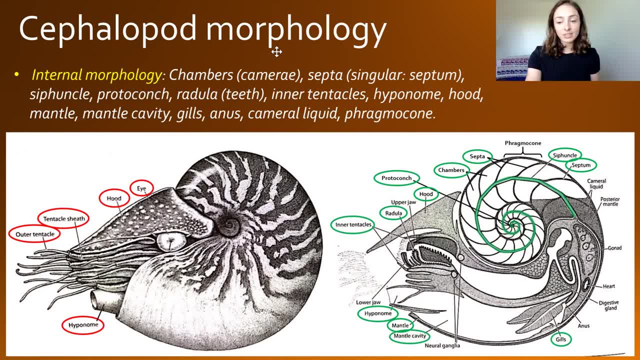 and then the mantle, the mantle cavity, feathery gills, the anus, carol liquid- which, again, like we talked about, is controlled by transport through the syphuncle and the phragma cone, which is basically the entire part of the shell, that includes all of the chambers except the living. 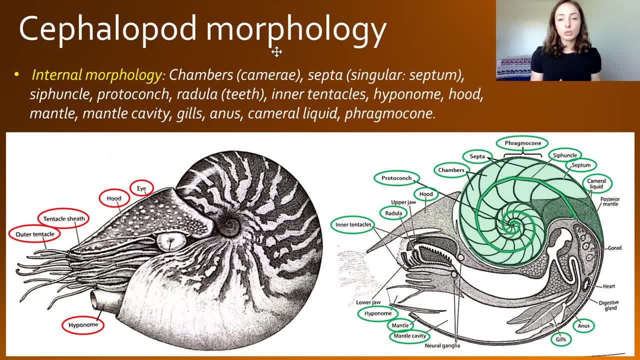 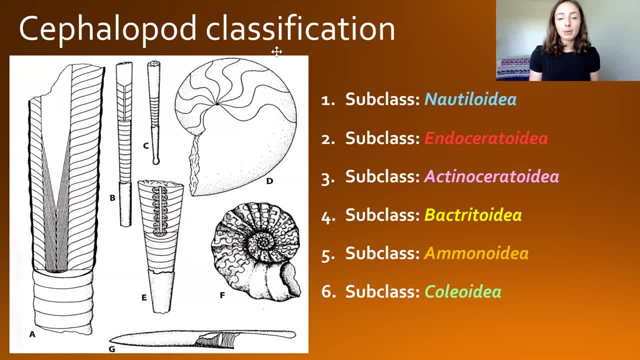 chamber, which is the chamber in which the animal currently lives. so the outermost chamber is the living chamber and the rest is the phragma cone. so now that we have general morphology out of the way, we'll talk a little bit about the six major subclasses of cephalopods, which includes 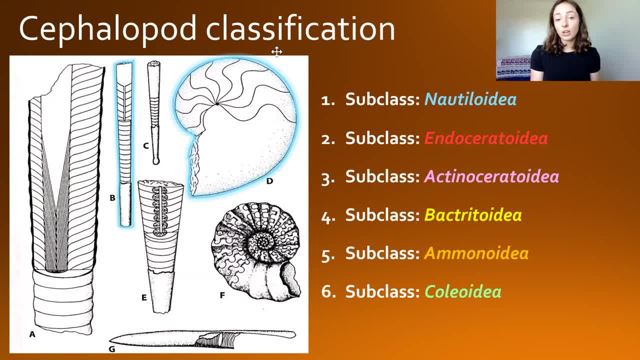 nautiloidia, which we've already talked about. some of the nautiloids which we talked about straight shelled ones, but they can also be plan a spiral or coiled in one plane, as shown here in figure two, and then we'll talk a little bit more about the other subclasses of cephalopods, which includes 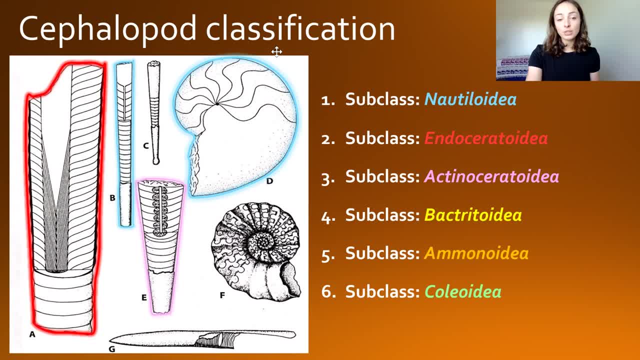 d, and then we also have endoceratoidia and actinoceratoidia, which are both straight shelled forms and both very large. however, they're different in that they have different cameral and syphuncular deposits. so, basically, cephalopods can have calcareous deposits within their camera or 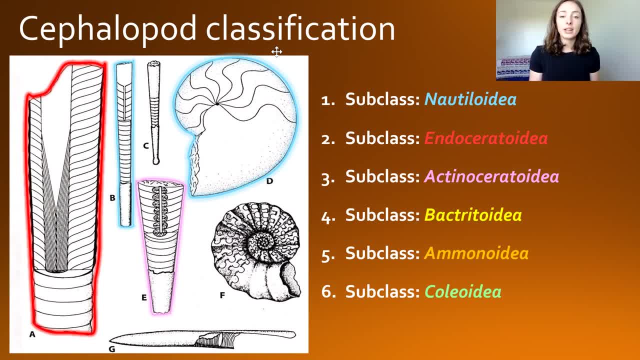 chambers and they can also have calcareous deposits within their syphuncle, and these are called cameral deposits and endosiphuncular deposits respectively, and we can see that the morphology of cameral and syphuncular deposits shown here on the endoceratoids and actinoceratoids are different. 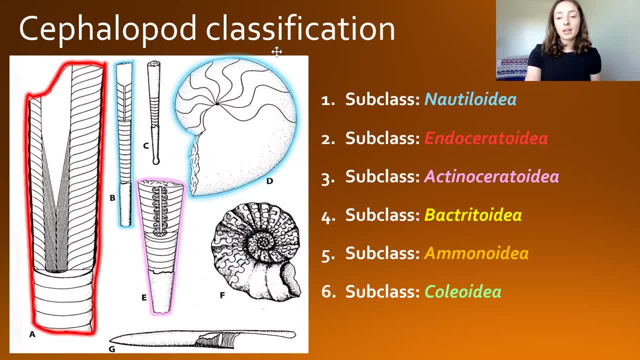 and that's how they can be told apart. additionally, we have the subclass factortoidia, shown here outlined in yellow, which is another straight shelled group, but these are very small in size and they have a globular protoconc, which is a distinctive feature for this subclass. 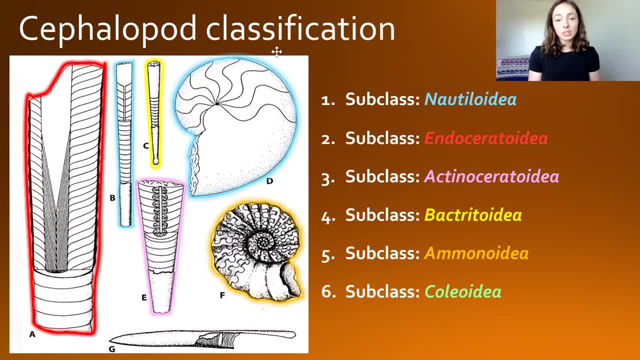 additionally, we have aminoidia, which is also something we mentioned earlier, the aminoids, which are major index fossils for the paleozoic and mesozoic phytophthene- and this is a very eras- and we'll talk a little bit more about their specific morphology in the next couple slides- and 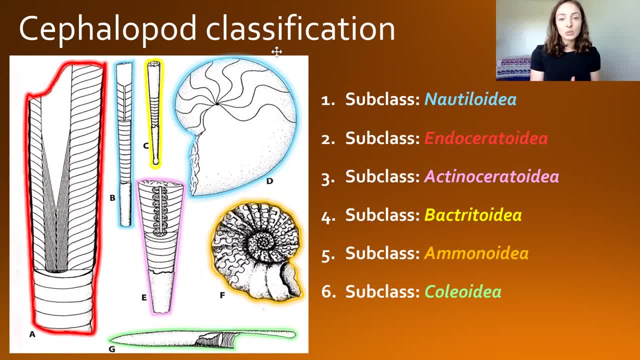 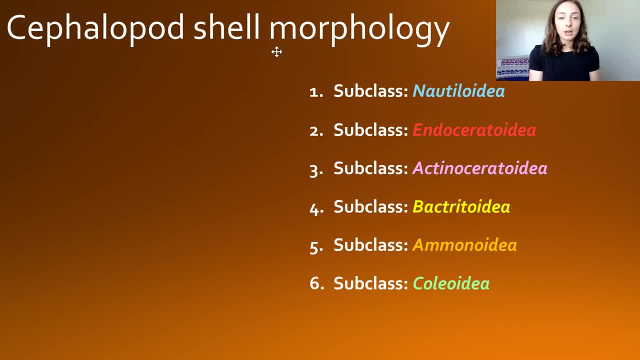 then, lastly, we have colloidia, which includes bulimnites, which can also act as really good index fossils during the mesozoic era as well. so, in terms of shell morphology, we already talked about the major kind of anatomical features that cephalopod share in general. but now i want to talk 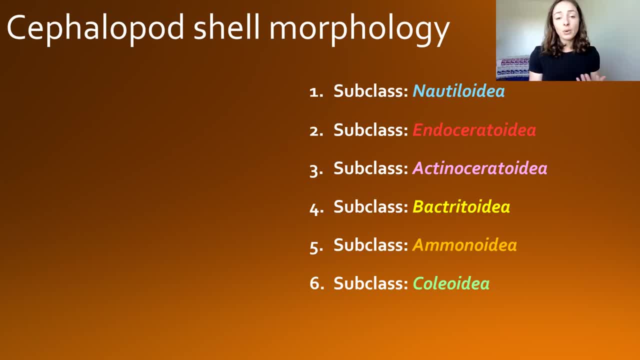 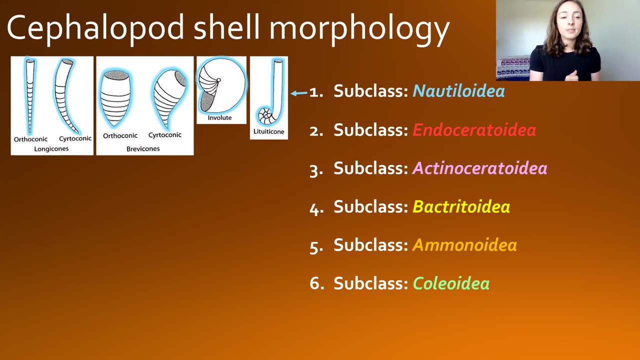 about different ways in which cephalopod shells can be coiled or can be straight, or can be slightly curved, etc. and so let's get into that. first, we have subclass nataloidia, which can have a variety of forms, such as straight shelled forms, which are called orthoconic, and slightly curved forms, which 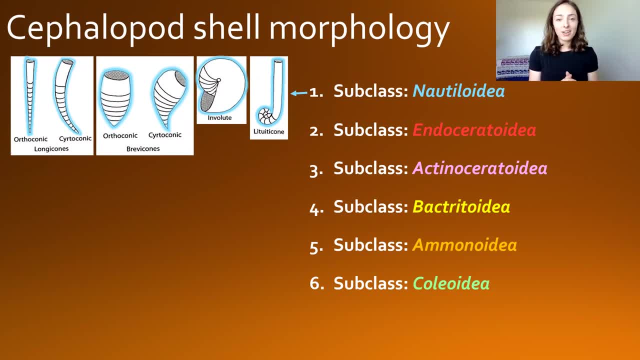 are called cerdoconic. i couldn't find a pronunciation online, so we're gonna go with cerdoconic, and both straight or orthoconic and slightly curved. cerdoconic shell morphologies can be classified in two different ways, and these include: 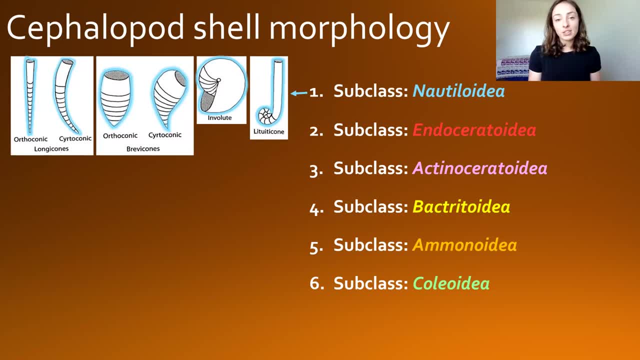 longicones and brevacones, and this just depends on, basically, the width of the shell. the brevacones are a little bit wider, as we can see, and then there's also coiled nataloids, such as latutocones, which are only coiled a little bit and then straight throughout the rest of the shell and 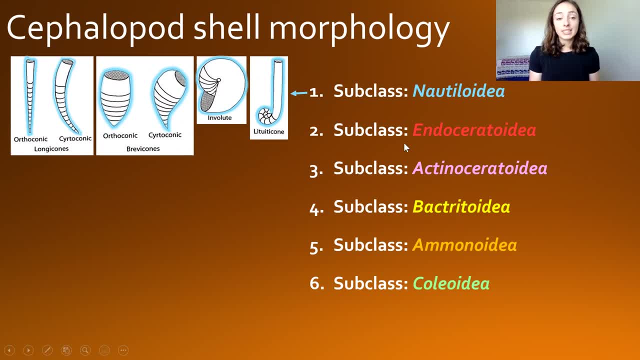 involute, planar spiral forms of nataloids, which are common forms today and, as we'll see later, the aminoids share similarities with this plan of spiral type of shell morphology. additionally, we have endoceratoidia, aptinoceratoidia and endoceratoidia, and endoceratoidia and endoceratoidia. 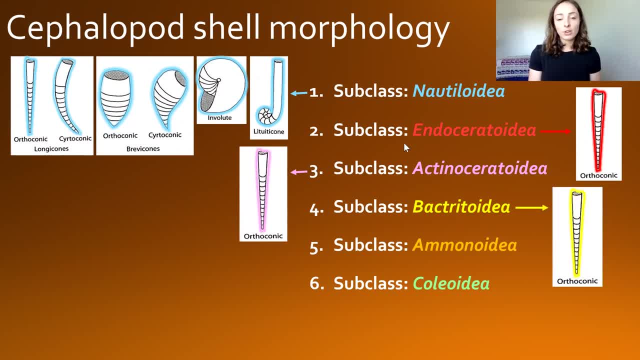 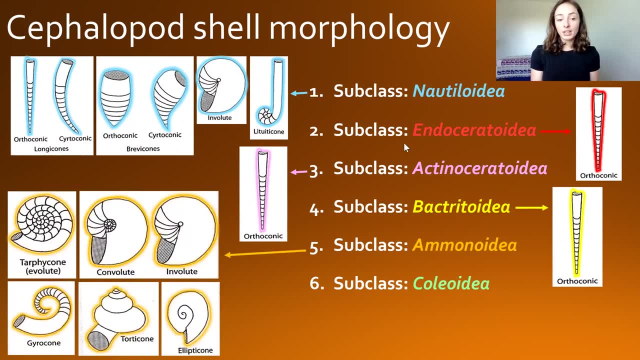 and bactritoidia, all sharing the orthoconic or straight shell morphology. then we get to aminoidia, which has a diverse variety of planar, spiral and trochospiral shell morphologies, and we'll talk more about these types of shell morphologies in a later slide, so don't worry. 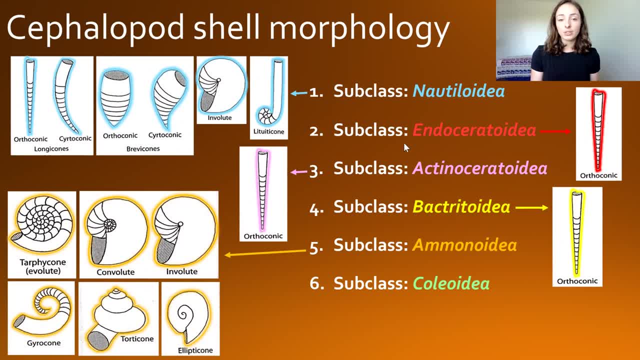 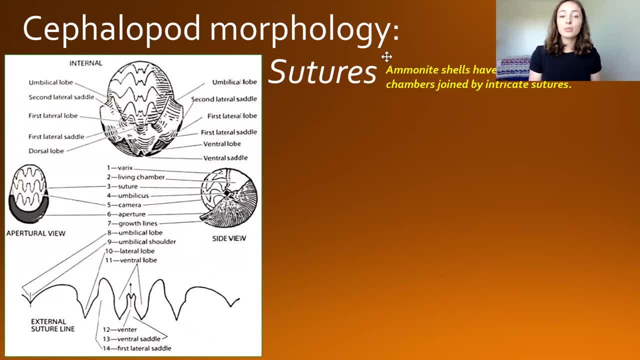 about those terms yet. we'll talk about those and identify and define those later on. lastly, we have colloidia, which is also another orthoconic group. so now we can get to looking at Aminoids. uterus- uterus are really important distinctive feature on aminoids. 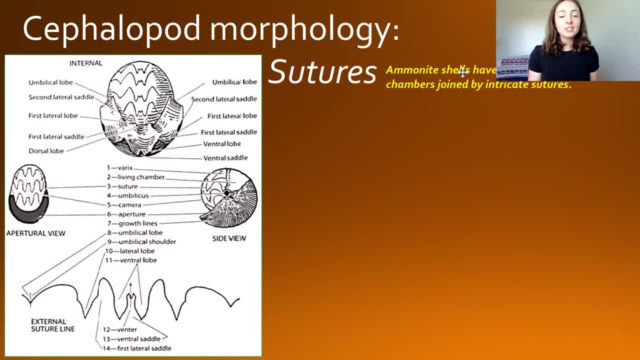 aminoid shells have chambers like all cephalopods, but the chambers on aminoid shells are joined together by intricate sutures and these sutures can be different in their pattern. but before we get to the main types of suture patterns, we need to talk a little bit about the terminology that 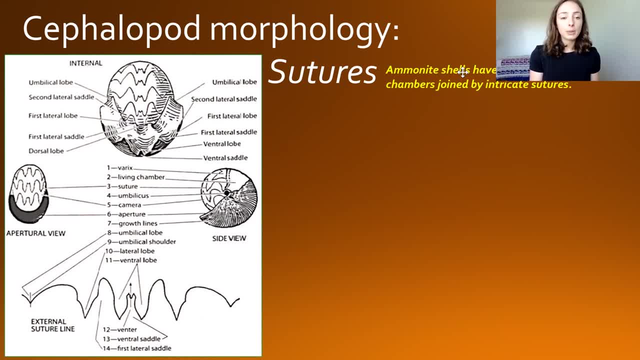 comes along with identifying suture patterns on aminoid shells. here we can see a figure showing in the top of the figure and at the bottom of the figure it's laid out so we can see the suture and each one of its saddles and lobes respectively. the saddles are basically the features that point. 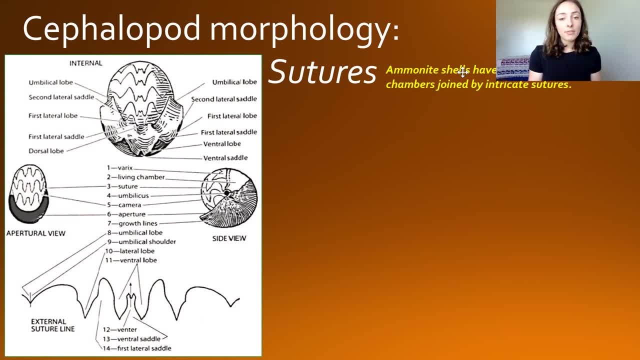 toward the head, and the lobes are the features in the suture that point away from the head. so if we label this, as we go from the center to the outer parts of the shell, we have the ventral saddle in the center of the shell which is pointing toward the head. then we have the first lateral 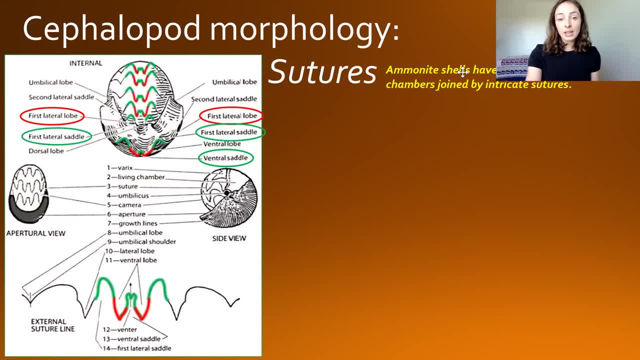 lobe pointing away from the head, then we have the first lateral saddle pointing toward the head again, then the second lateral lobe, then the second lateral saddle, and so on until you get to the umbilical lobe, which is the last lobe of the structure, as that gets to the center of the shell. 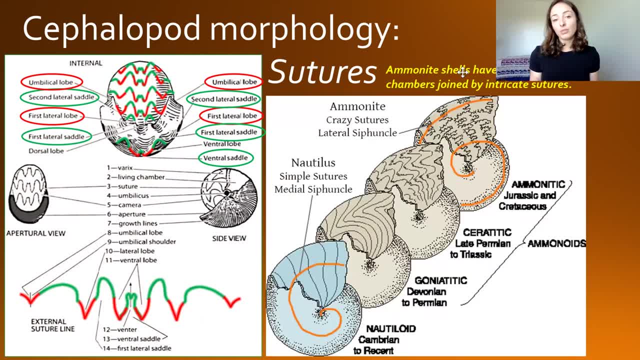 or the umbilicus of the shell. so now let's look at some different types of suture patterns in aminoids throughout time. first, we have a nautilus, shown at the bottom left of this slide, which has a central hole in the nautilus, and that is where the nautilus is located. that's where the shell is. 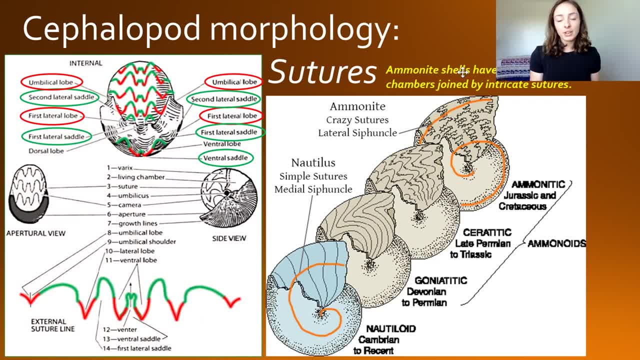 its simple suture pattern, as well as its medial syphuncle, which is another difference between nautiluses and aminoids is that it has a medial syphuncle that penetrates through the center of each of its septa. However, aminoid shells typically have a more ventral. 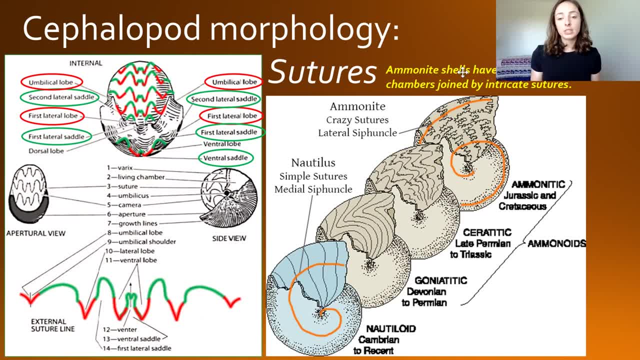 or outer syphuncle that goes through the outer parts of each of its septa, And we can see this by the orange line showing where the syphuncle would be in each shell. Now, if we look at the nautilus sutures, 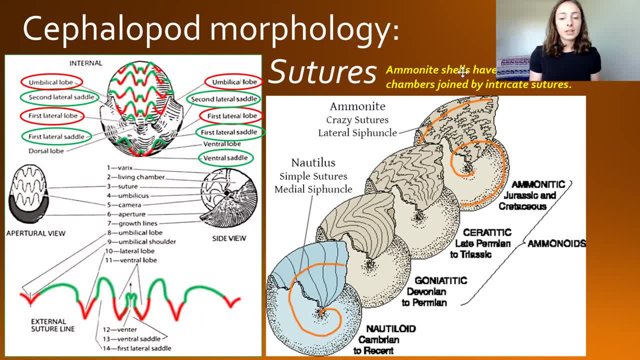 we can see. they're very simple, kind of straight. a little bit of curve in there, but nothing crazy in the nautiloid shells. However, as we move to the three aminoid shells, we see that the suture patterns become more complex. 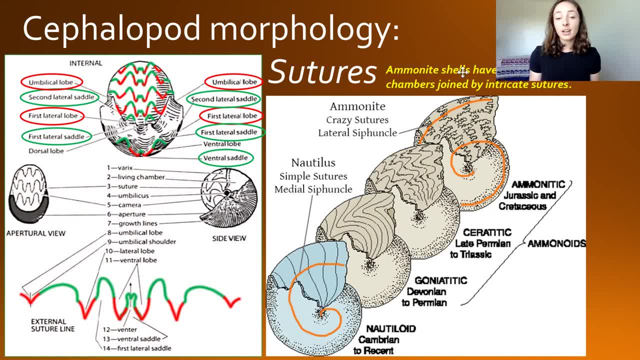 As we can see, the first step toward this complexity is in the goniotidic suture patterns. These goniotidic suture patterns were most common from the Devonian to the Permian period in aminoid shells, Then, as we move to the late Permian, to Triassic. 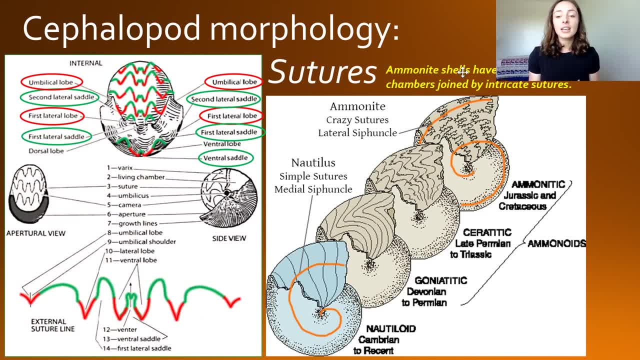 the most common suture pattern is a little bit more complex than goniotidic, and that is the serotidic suture pattern, which has crenulated lobes, as we can see in the picture. Then we move to the ammonitic suture patterns. 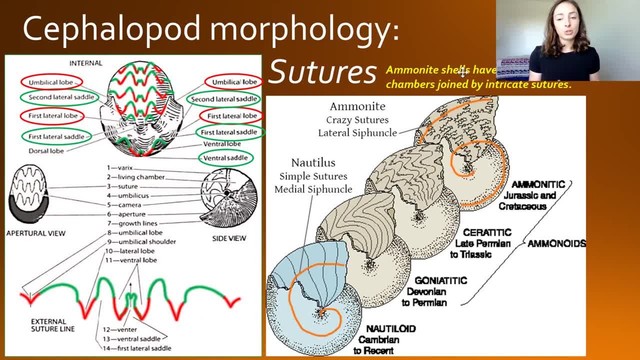 which are just really crazy kind of dendritic, almost suture patterns that were most dominant during the Jurassic and Cretaceous, at the peak of dominance and complexity for the aminoids. And this is when we see the most complex suture patterns. 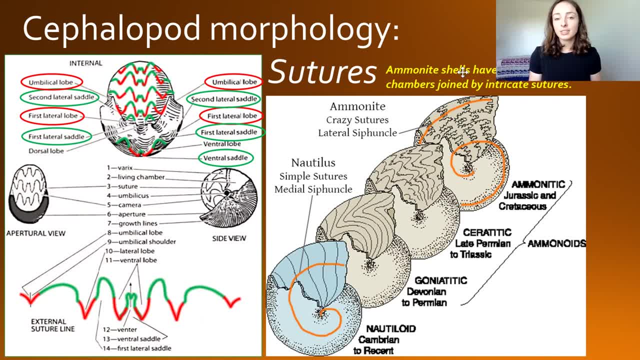 This evolutionary trend in suture patterns and aminoid shells is not only really aesthetically pleasing in the fossils that we can collect and then make into jewelry and stuff, but it's also really helpful for biostratigraphy throughout the Devonian to the late Mesozoic. 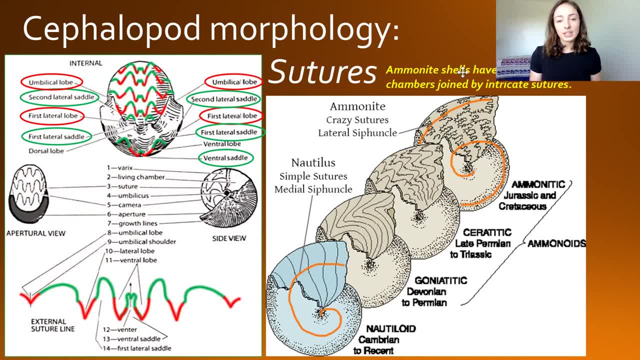 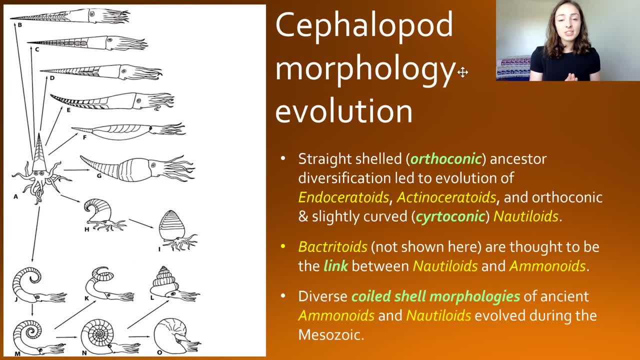 We have all of these really intricate designs in the sutures of these ammonites that evolved rapidly, with enough steps that we can tell exactly where we are, depending on the suture patterns in the aminoid shells. Now let's talk a little bit. 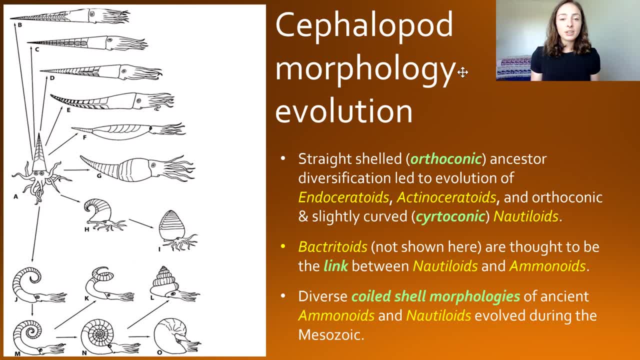 about cephalopod shell morphological evolution. So, like we already talked about, most of the subclasses do have orthoconic or straight shells, such as the endoceratoids, the actinoceratoids and a lot of the non-endoceratoids. 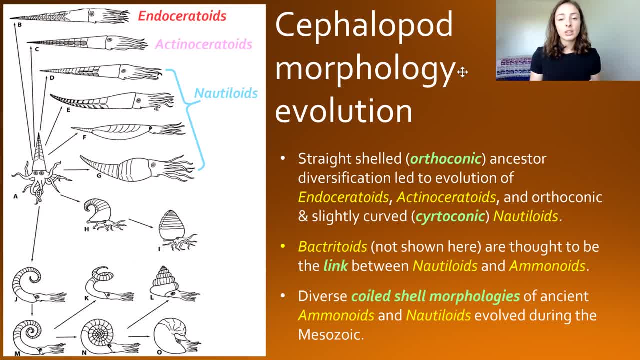 and a lot of the endoceratoids, and a lot of the endoceratoids, which also include slightly curved or cerdochonic shells, and bactertoids, which are actually not shown on this figure, also have orthoconic or straight shells. 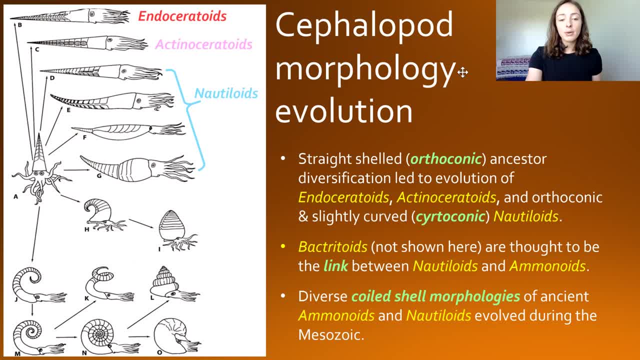 And this group is thought to be the link between nautiloids and aminoids. However, once we get to later nautiloids and aminoids, we do see that shells begin to coil more than orthoconic and cerdochonic forms. 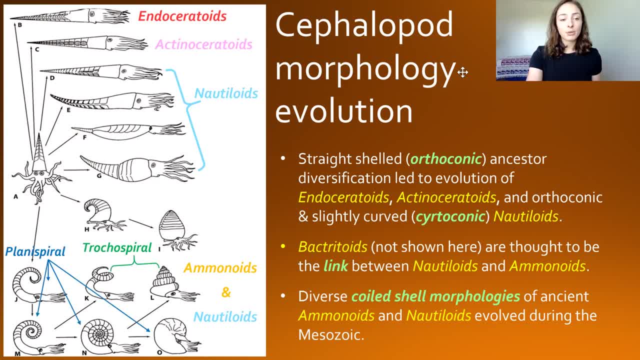 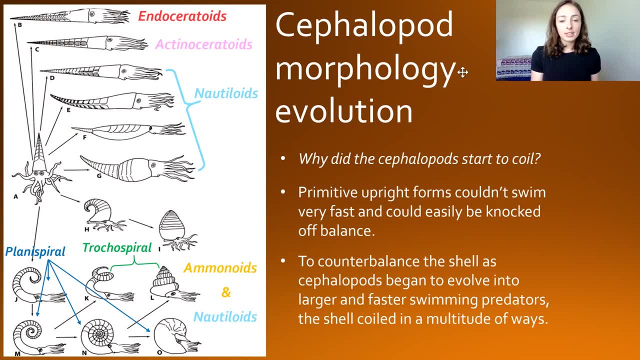 And within these coils we have both trochospiral and planospiral forms. So why did cephalopods start to coil? Well, primitive upright forms such as figure A in this image couldn't swim very fast and could easily be knocked off balance. 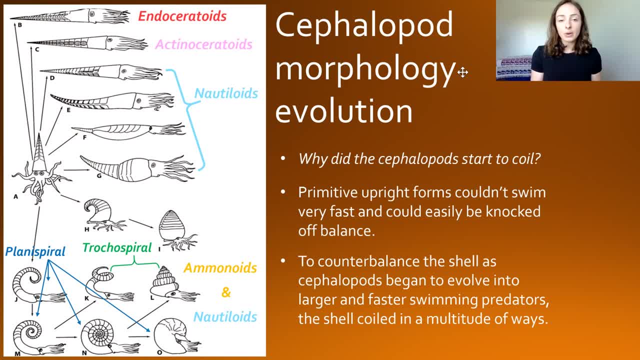 based on how their shell was shaped and how they floated. However, later, to counterbalance the shell and allow cephalopods to swim faster- and actually, instead of having the upright orientation, have a sideways orientation so they can swim faster- cephalopods began to coil in a multitude of ways. 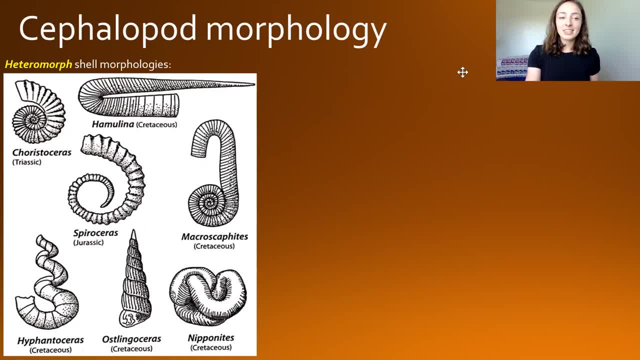 as they diversified And some ways were pretty funky. And these funky shell morphologies of cephalopods are called heteromorphs. Heteromorph shell morphologies, as shown in this figure, are all different morphologies of aminoids. 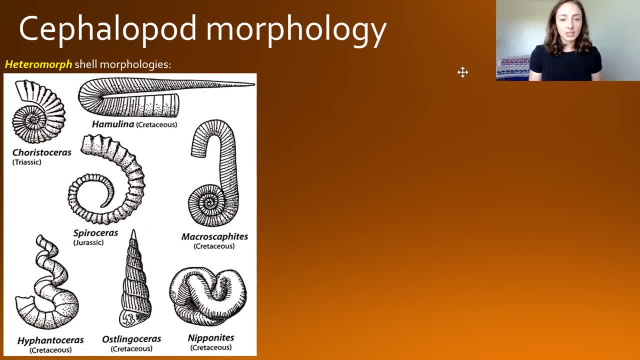 which went through a series of radiations through the Paleozoic and Mesozoic eras And, as we can see, these shell morphologies include hamatocones, which are shells that form two or more straight shafts. Then we have encyclocones. 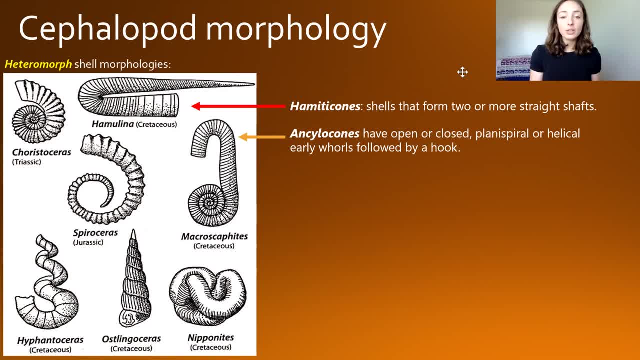 which had open or closed planospiral or helical early whorls that were followed by a hook at their end, And then we had torticones which had helical whorls, and then some loosely formed torticones which are shown here by the genus Hyphentoceras. 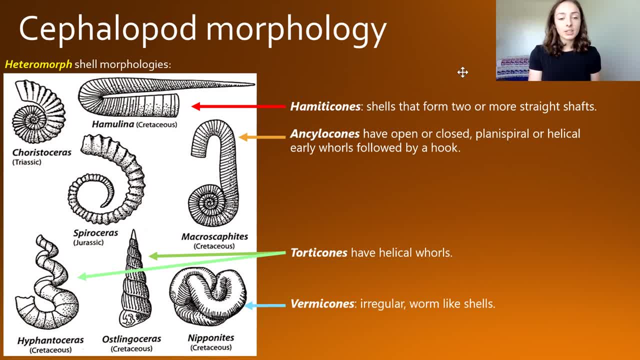 Then we had vemicones, which were irregular worm-like shells, And finally we had some planospiral forms, which were more run of the mill for ammonites, And we'll talk about the different forms of planospiral shells here. 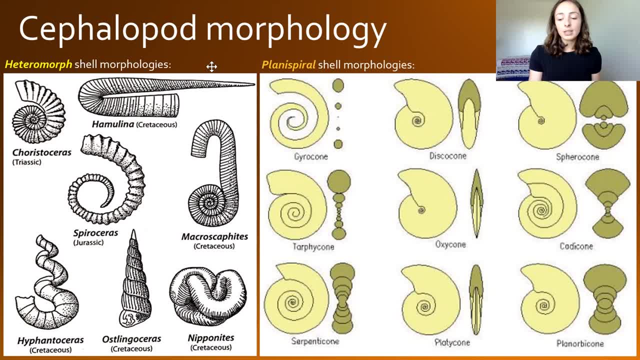 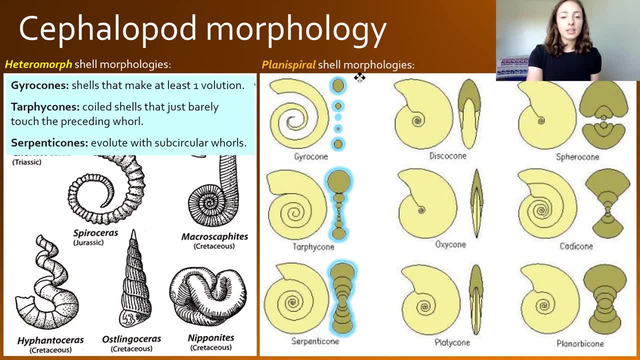 So here we see different planospiral morphologies for ammonites, and we can see these include gyrocones, which are shells that form at least one volution, but their coils don't necessarily touch. Then we had tarphocones. 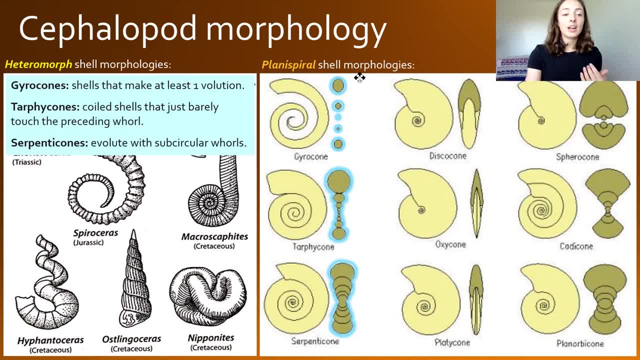 in which their coils did touch, but just barely. And then we had serpentocones, which still had sub-circular coils, but they were compressed more by touching each other more heavily. but they weren't quite involute yet, They were still evolute. 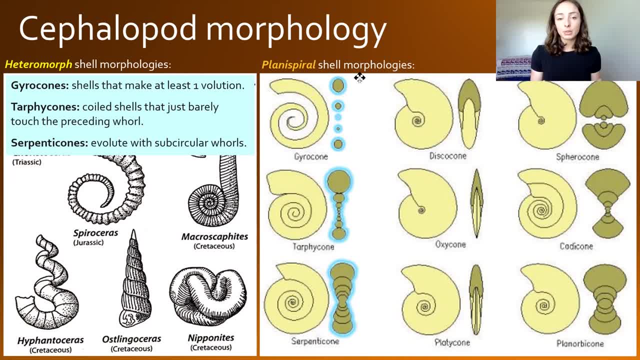 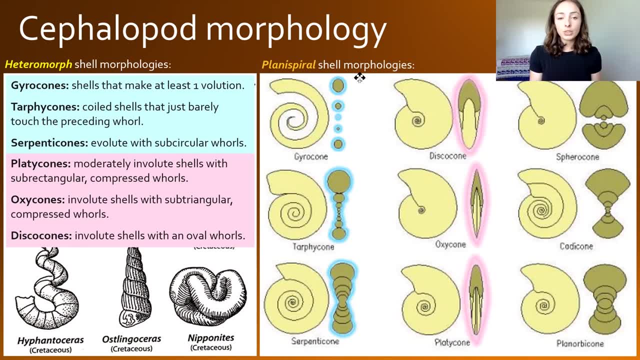 meaning their inner coils still showed They weren't covered up by the subsequent coils. However, then we have platycones, oxacones and discocones. We have discocones at the top here with involute shells that have oval whorls. 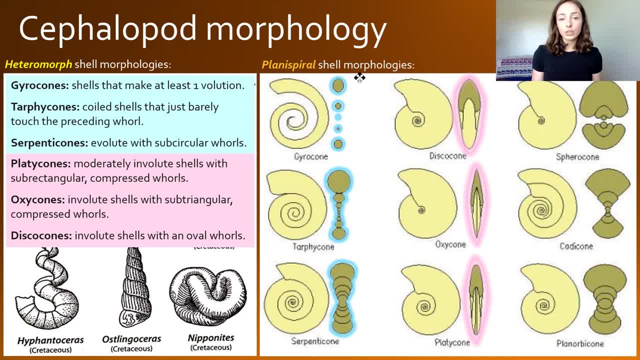 So we can see those inner coils don't show very well because they're involute. The subsequent coils are covering them up. Then we have oxacones with sub-triangular compressed whorls, As we can see, this one's more compressed. 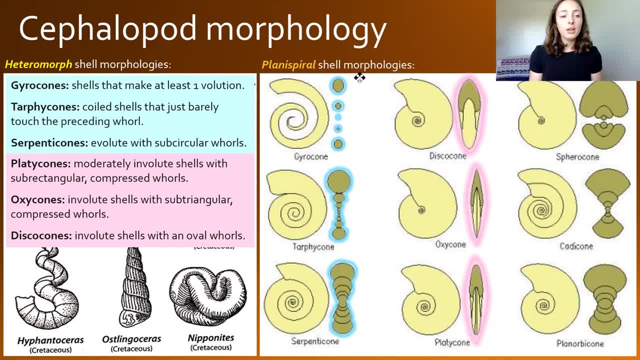 and looks like it would be a little bit more streamlined and a faster swimmer. Then we have platycones, or platycones which are moderately involute shells, So they have some of their inner coils shown, but some are covered up. 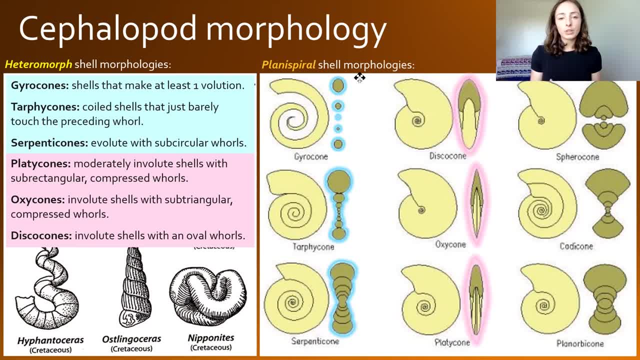 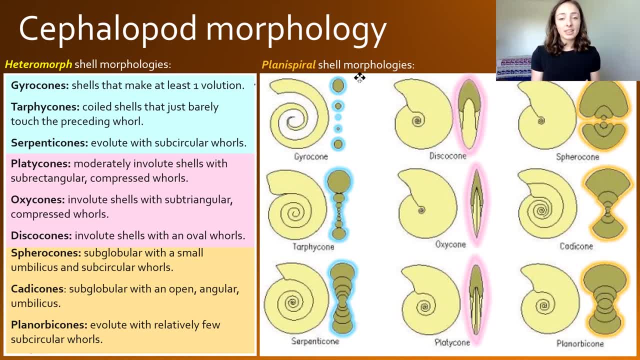 and these have sub-rectangular compressed whorls, So they were also likely pretty streamlined. Then we have spherocones at the top right here which are sub-globular and are very thick and probably wouldn't be the fastest swimmers. 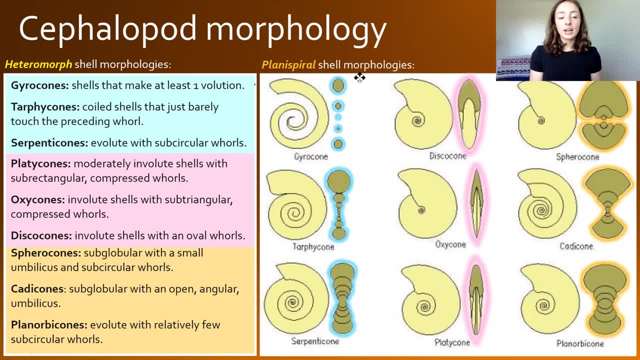 And they also have a very small umbilicus. And then catacones are also sub-globular, with an open angular umbilicus. And then planorbocones are the last shell type we see at the bottom right here, and these are evolute. 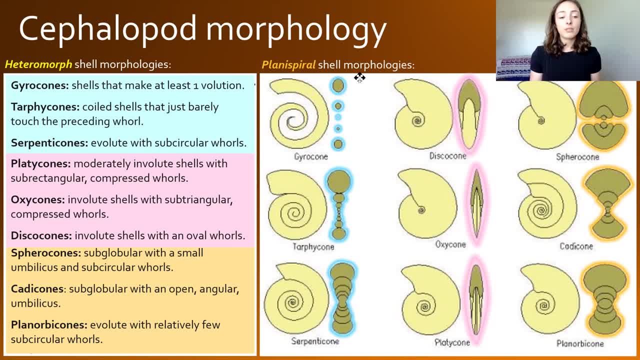 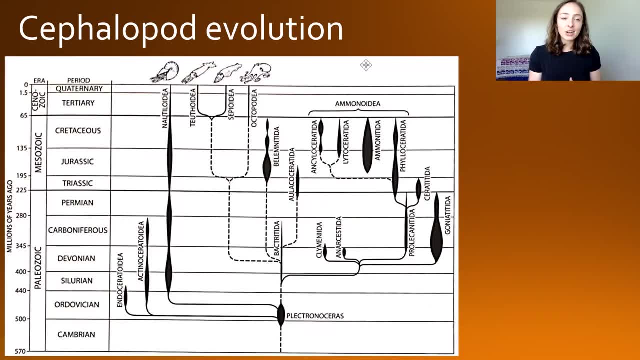 So their inner coils are shown and not covered up, and these have relatively few sub-circular coils, So they're similar to the serpenticones, but they have less coils. So now let's talk about cephalopod evolution. Cephalopod evolution can be shown here by this chart. 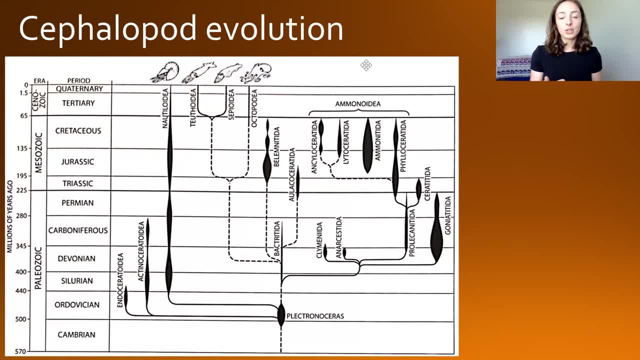 We'll start at the bottom in the Cambrian and go all the way up to the quaternary or now as we move through the different evolutionary events in this timescale. First we have the earliest cephalopods or Plectronoceras evolve. 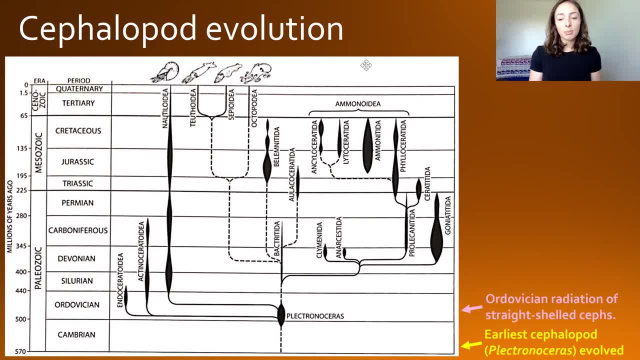 And Plectronoceras led to the evolution of straight-shelled cephalopods during the Ordovician radiation shown by the diversification. So we have the evolution of endoceratoidia and actinoceratoidia, as well as nautiloidia. 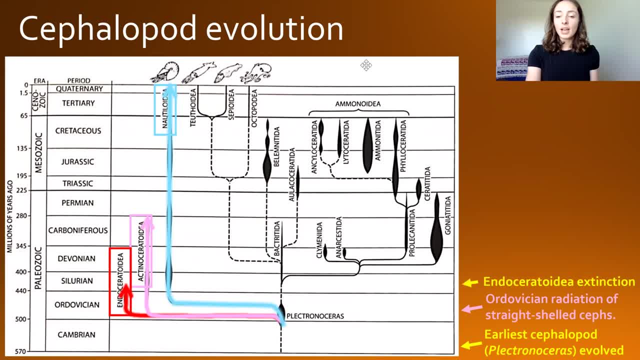 which, as we see, ends up surviving until the present. And then we have endoceratoidia go extinct during the Silurian, Then we have Bactritoidia and Aminoids, or Aminoidia, evolve during the Devonian. 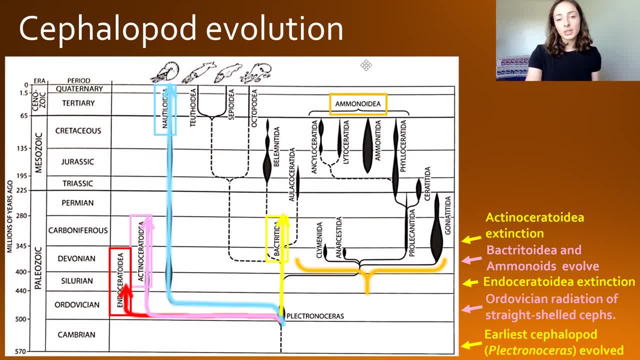 as shown here in yellow with Bactritoidia and here in orange with the Aminoidia. Then we have actinoceratoidia go extinct during the Carboniferous period. Then we have cephalopods decline the end Permian due to the Permatriassic extinction. 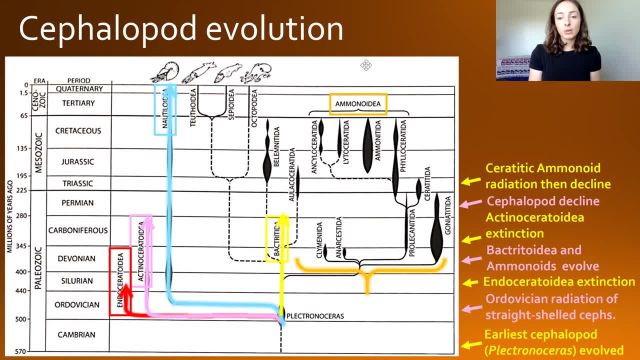 then a subsequent radiation of Ceratitic Aminoids during the Triassic period, But then during the late Triassic, during the in Triassic extinctions they had, the Ceratitic Aminoids declined just before the Jurassic Cretaceous radiation. 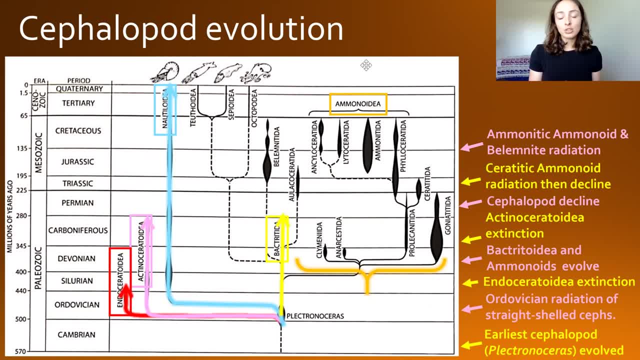 of Ammonitic Aminoids, So Ammonoids with Ammonitic suture types, and then Belemnite radiation during the Jurassic Cretaceous as well, making Ammonitic Aminoids and Belemnites very good index fossils for the Mesozoic.